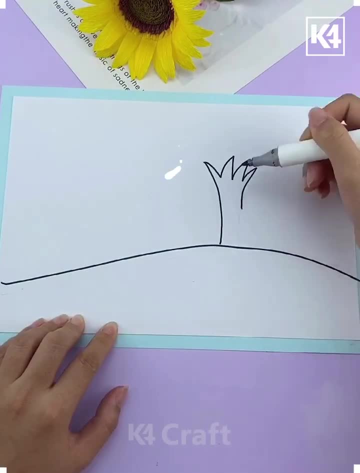 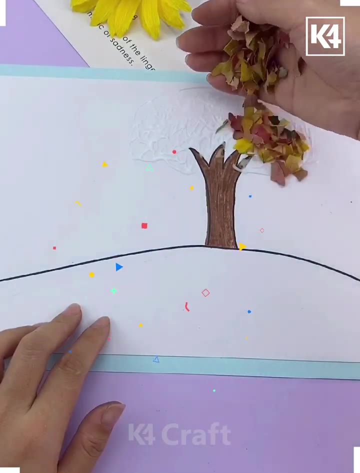 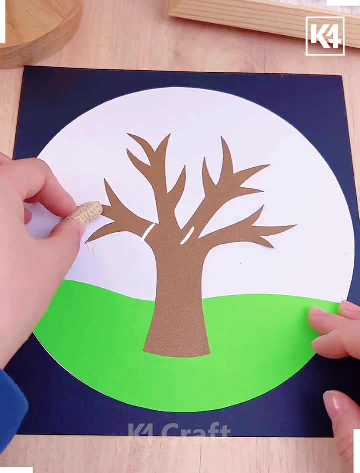 hello everyone. a very good morning to one and all. today we are drawing a painting with real leaves and flowers and making beauty out of garbage. firstly, we made a tree with the crushed leaves on a white background, a greeting card, stick a brown color tree shape on it and take some. 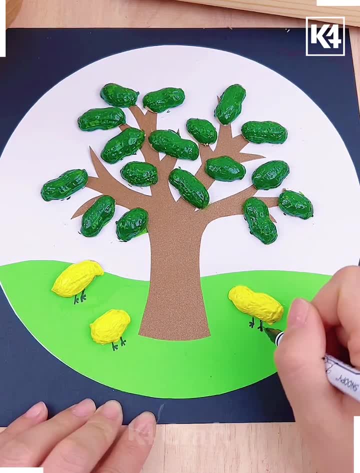 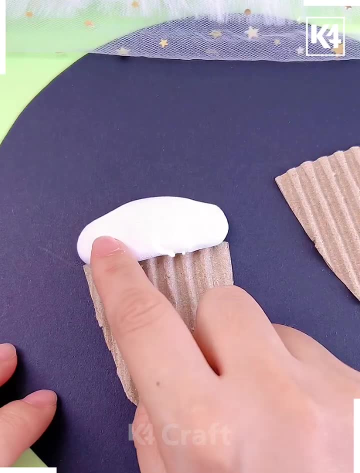 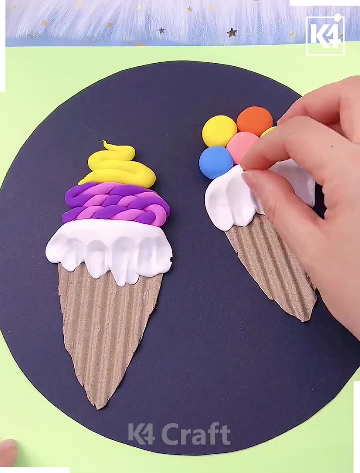 ground nut shells and stick them as you like and paint them with green and yellow color. now, using two cardboard pieces and modeling clay, we are making two ice cream cones, as shown. so on the top, as shown, and give them toppings as you like, take a tool and dip in the red color. 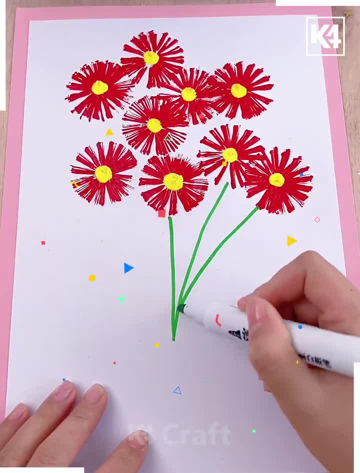 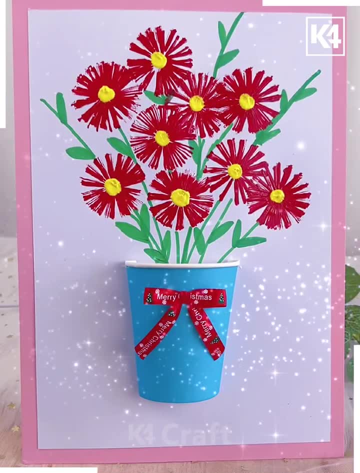 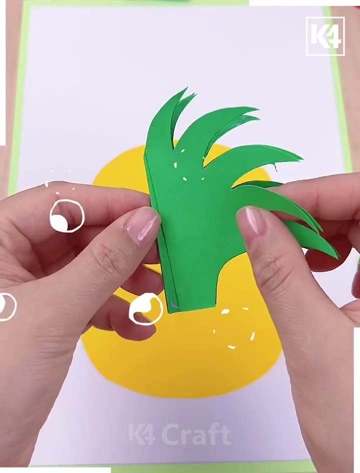 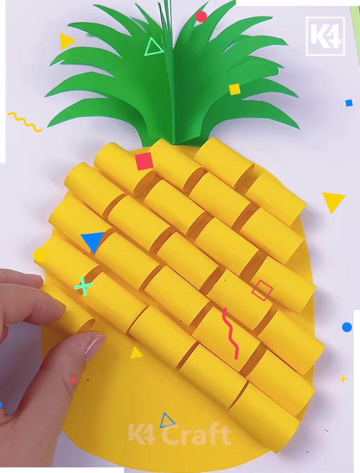 and make as shown the flowers and give green lines and leaves for the flowers. stick a paper glass and give it a bow. next, make a yellow colored paper like shown in the shape and cut a green color paper by folding as shown and cut the paper according to the line drawn on the stick. so, on the top, as shown, take a small paper pieces by folding and 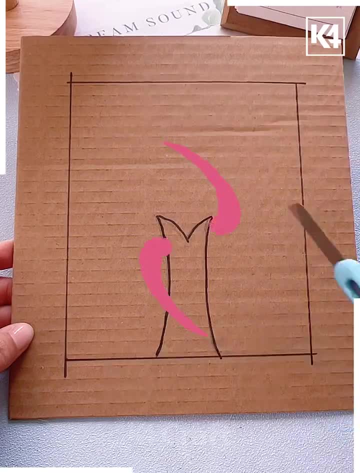 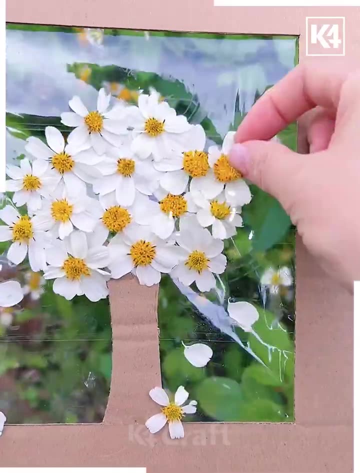 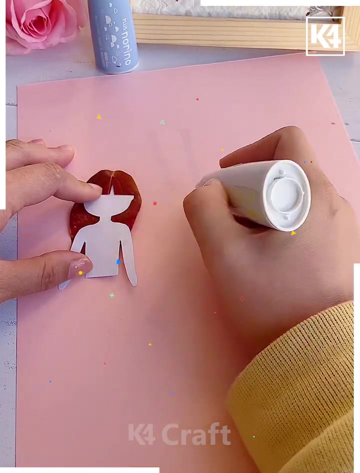 sticking like as this. take a photo recognizer cardboard with a wooden color on the middle and paste transparent tape on the back side and stick different flowers onto it as you like. next we are making a barbie girl. take a dried leaf, cut it as shown and cut the yellow colored barbies like shown and make mar inauguration. making akellinger barbie. 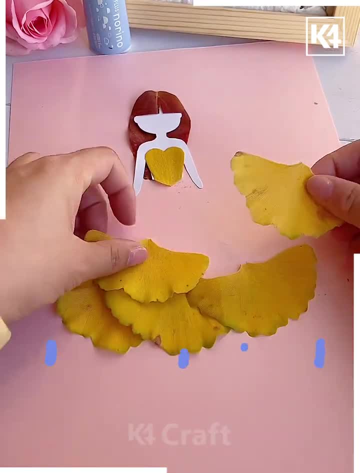 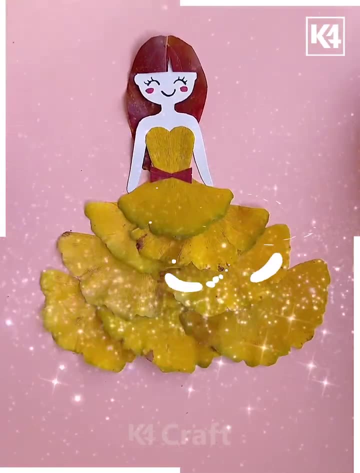 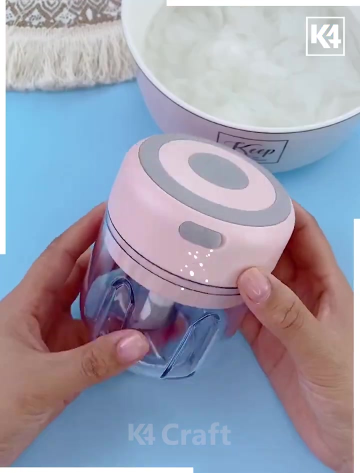 make a face part should be shown and stick pencil wastage like a flowy gown to the Barbie girl and give a bow in the middle. magic angel is ready. take some small flowers with the neat alignment, place them in a book. next close the book and leave it. next soak some tissues in water and grind it well and mix it in. 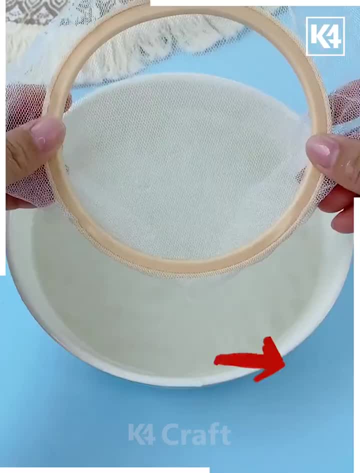 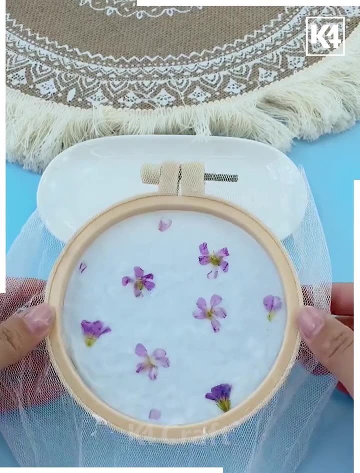 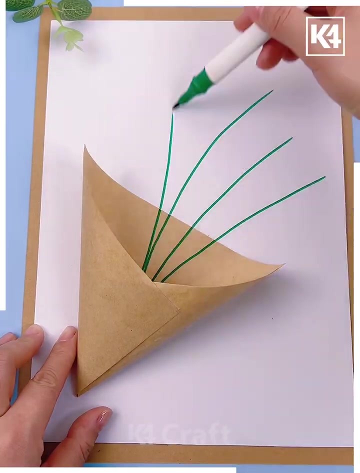 water thoroughly. take a net type cloth with a clip to it and filter the filter, the mixture from the ball. now place the flower previously stored in a book on that end right with the help of hand pan, we got beautiful arts in different way. next, fold a brown colored paper as shown and stick it to a paper and draw lines. 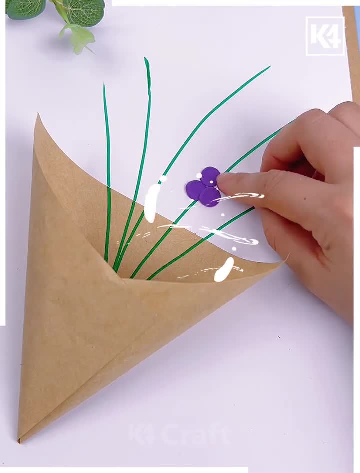 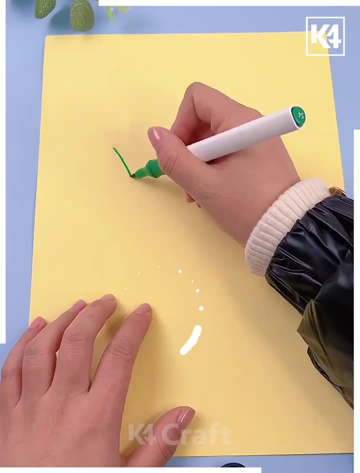 from the brown sheet to the white sheet and with the green sketch, and make rounds on both sides with modeling clay as shown and give it a bow. take a yellow colored background shade, draw a freehand line, ash like and make flower shapes with the care of your hand and give it a bow.